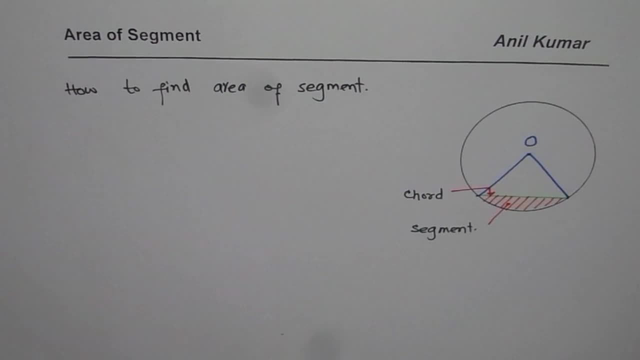 Then what do I get? In this case you will see: 1, I get a sector. Let us say the chord is A to B. So in this particular case I get two things: 1, I get a sector. Let us say this angle is given to us as theta. 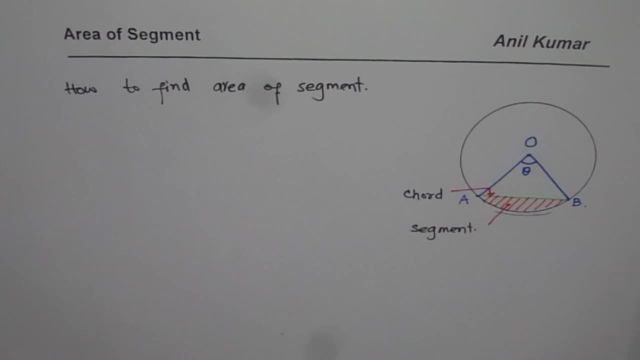 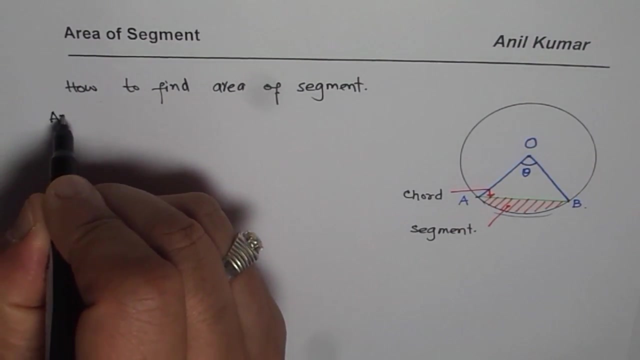 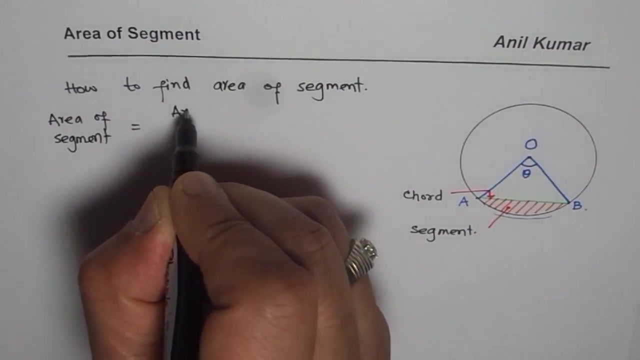 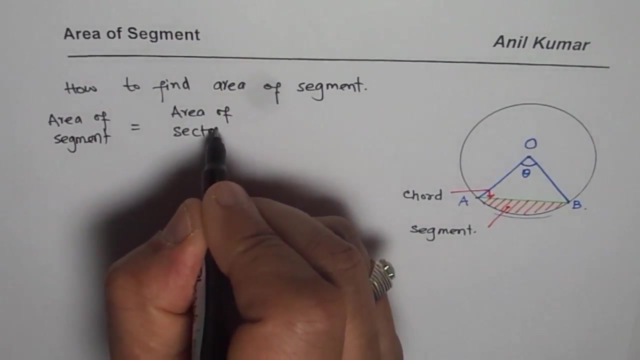 So in that case, what I can say is that the area of segment should be equals to, let us say, area. So the area of segment should be equal to area of the whole sector that is called the sector. take away, area of triangle. 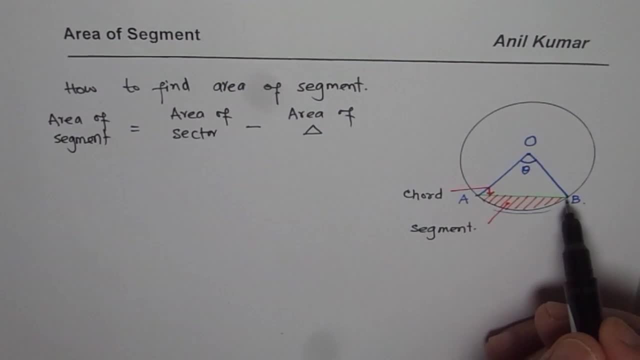 Do you get the point? So if I take away the whole area of sector, if I take away the area of triangle from the area of the sector, I get area of the segment. That is how you actually You can actually find area of the segment, right? 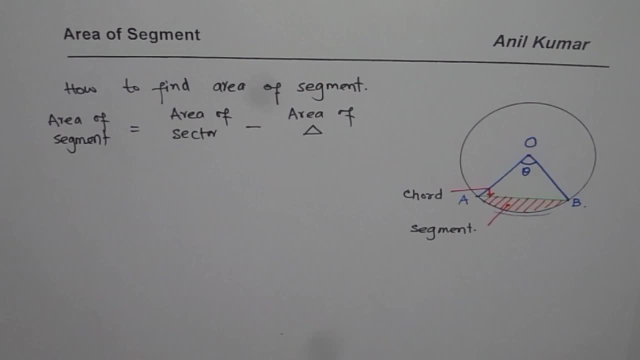 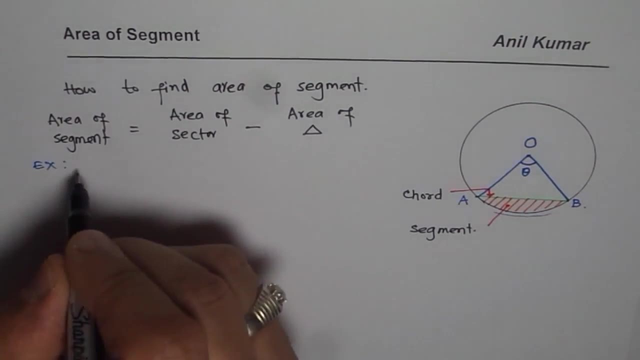 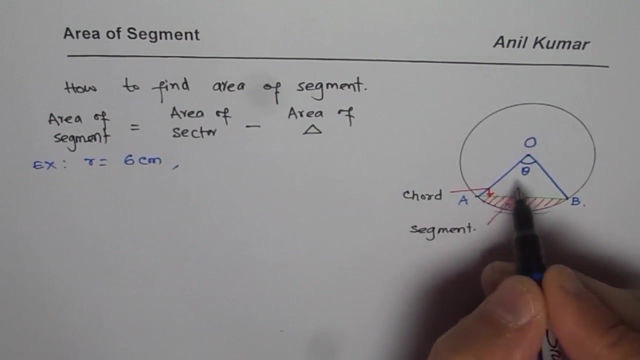 So if we are given some values for radius and angle, we can easily find this. So, as an example, let us take up an example now. So let us say radius is 6 centimeters, okay, And let us take this angle, theta, as 120 degrees. 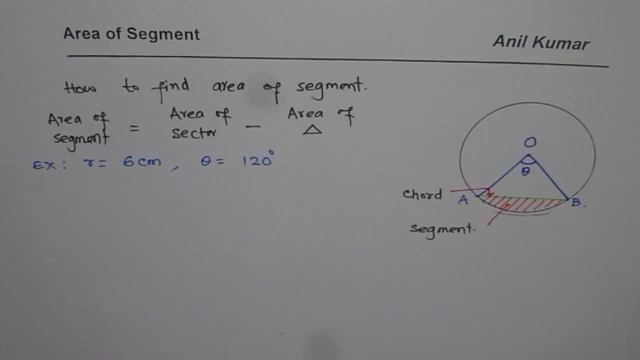 So if radius is 6 centimeters, Let me write down here 6,, and this is 120 degrees. in that case, how are you going to find area of the sector? So that is the question for you Now. can you tell me how? 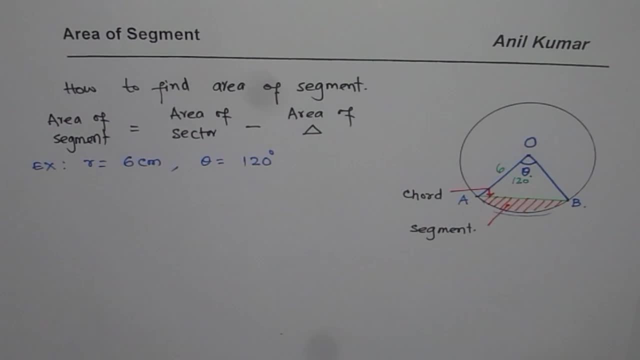 It is not that easy, right, Okay? so let us try it out. Area of the sector is ratio of total area to the one which is enclosed by the given angle. So we can say area of sector is equal to area of the segment. 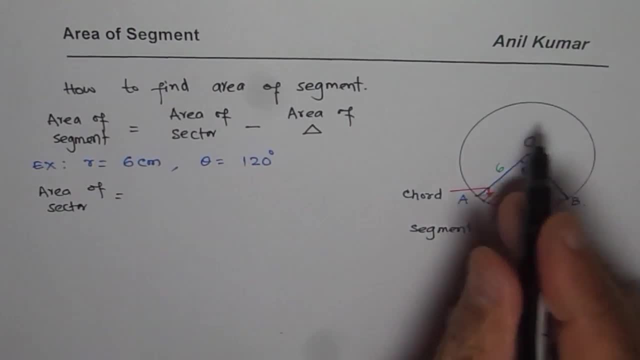 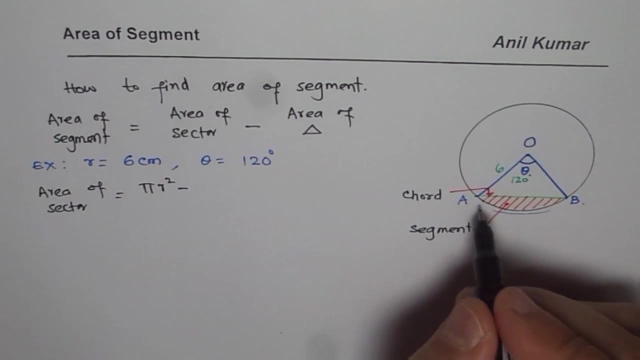 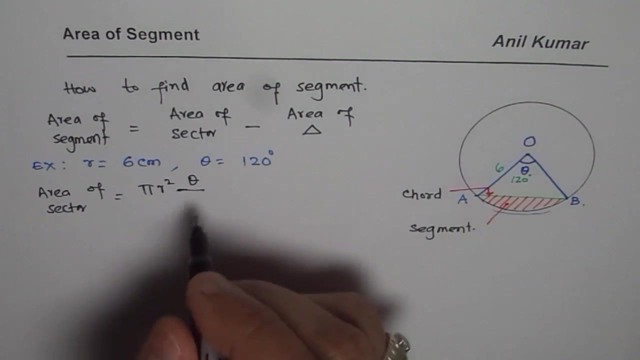 So the area of sector is circle area which is pi r square minus. I mean pi r square area of the sector. we are finding that area times theta divided by total angle, And since we are given angle in degrees, 360 degrees right. 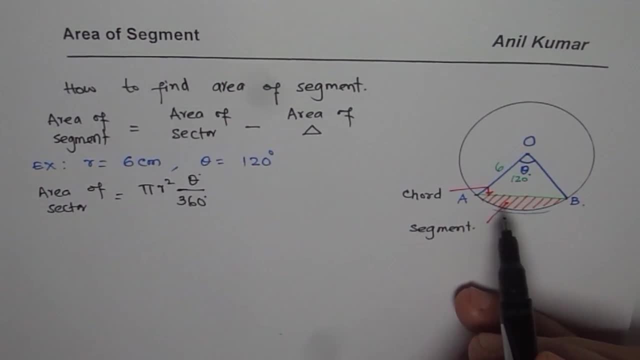 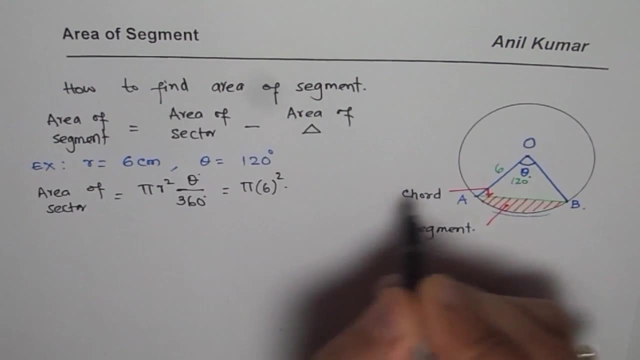 So it is a radius, It is a ratio of the angle enclosed right. So in our case we are given radius of 6, right. So we can write this as: pi 6 square angle is 120 degrees divided by 360 degrees right. 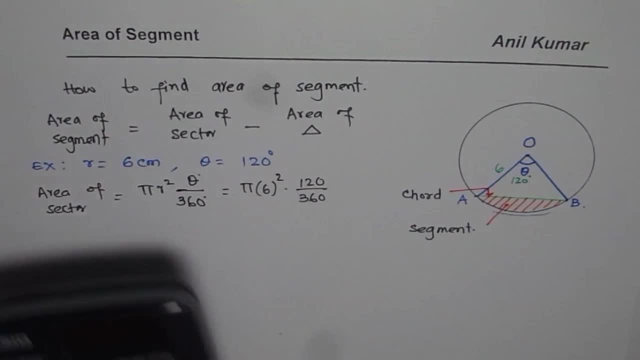 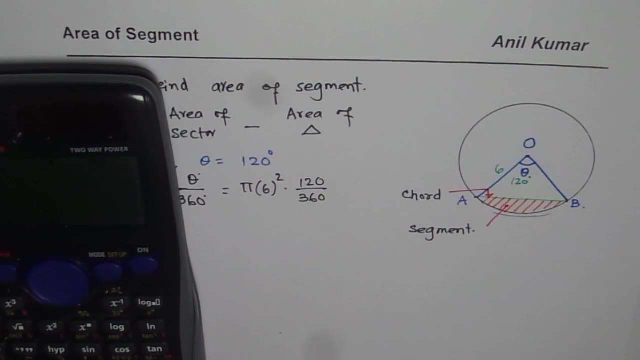 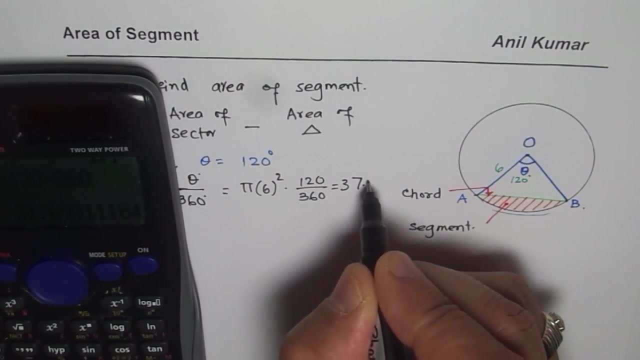 So that gives us the answer right. So we can use calculator to find the answer. So we have pi times 6 square. let us write 6 square and then times 120, divided by 360.. So that gives us 12 pi, or in decimals it is approximately 37 point. let me write 7: 0, okay. 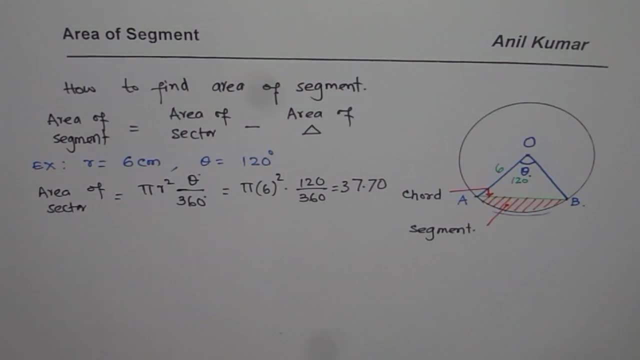 So I just round it to two decimal places. So that is the area of the whole sector. Now from this area I have to take away area of triangle. How to find area of triangle? That is a big question. right, To find area of triangle we may use a bit of trigonometry. 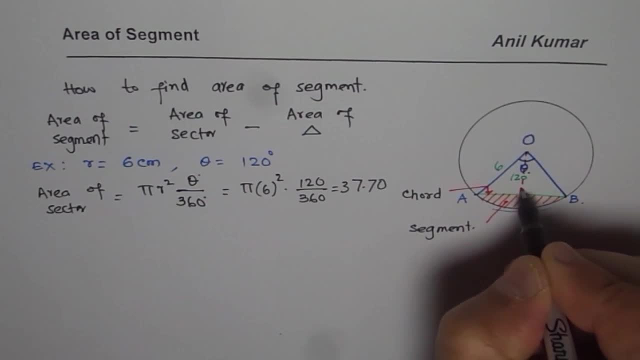 So what we need to do here is drop a perpendicular. So if I drop a perpendicular, then since these two sides are equal, these two sides will also be equal, correct? So let me say from O: I have a point P here. 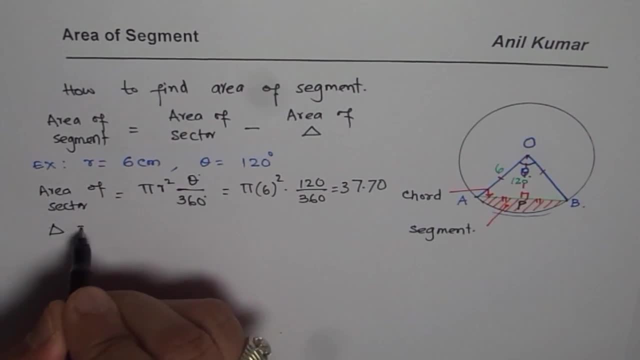 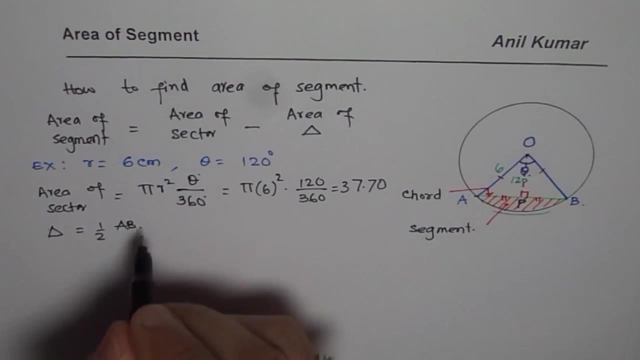 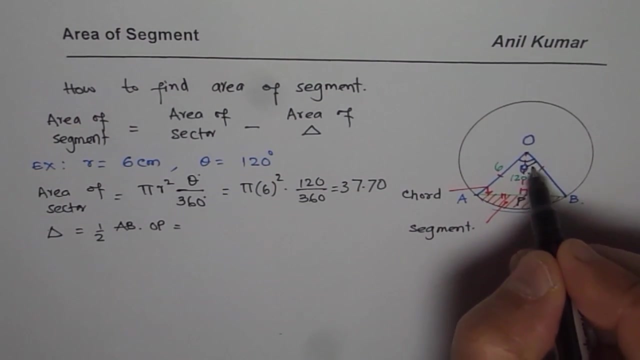 In that case, area of triangle. so we are looking for a triangle. It is half base, which is AB times the height, which is OP. Now we can use trigonometry To find this angle. Now half of this angle is here and half is on that side. 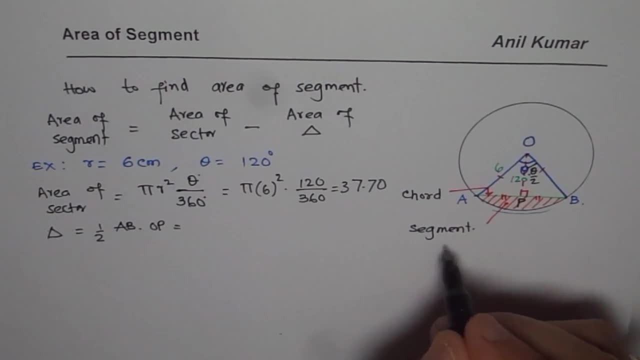 So using this half of the angle, which is theta by 2, let me write a general expression first- We can find what AP is right. So AP is opposite to half the angle right, Which in this case half of 120, 60 degrees right. 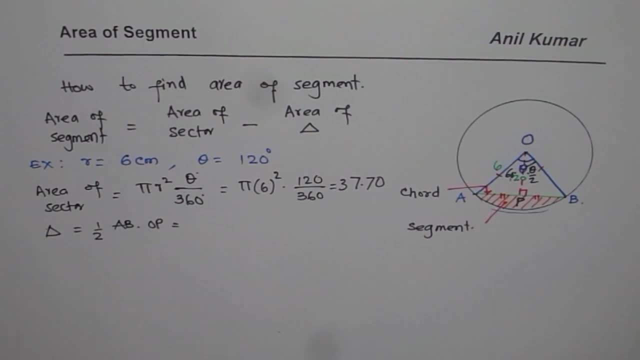 So I want to write 60 degrees on this side, okay? So in that case we know AP over hypotenuse 6 is equal to sine of 60 degrees, right? Therefore, AP is equal to 6 times sine of 60 degrees in this case, correct? 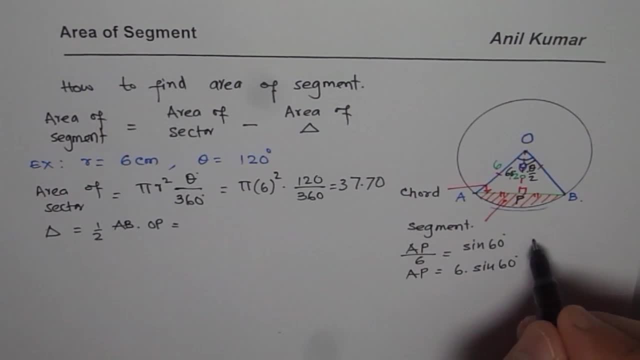 As far as OP is concerned, we can write OP over 6,. let me write it like this: is equal to cos of 60 degrees in this case, right? Therefore, OP equals to 6 times cos of 60 degrees, correct? 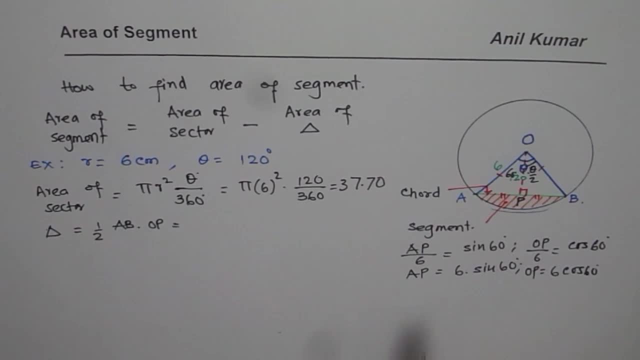 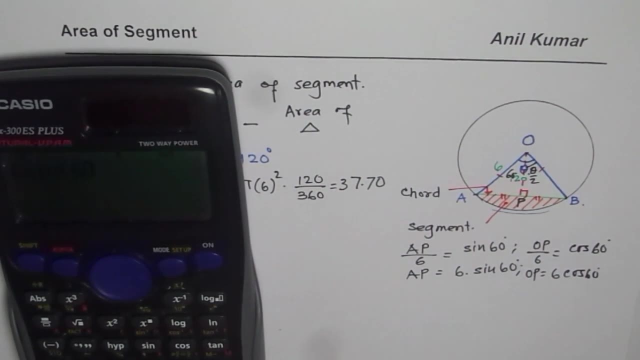 So likewise we can get both these sides. So let's get solve this right. 6 times sine of. we can use special triangles also to find this answer right. So 3 square root 3, okay. or let's convert to decimals, okay. 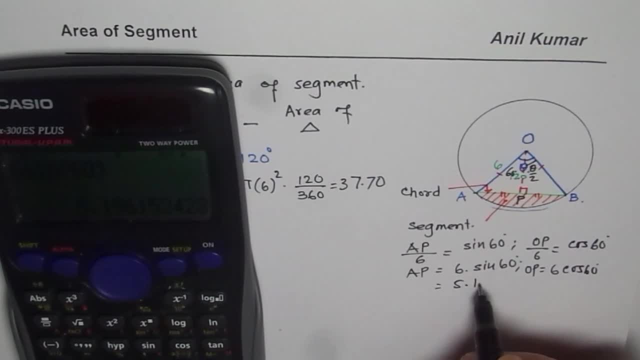 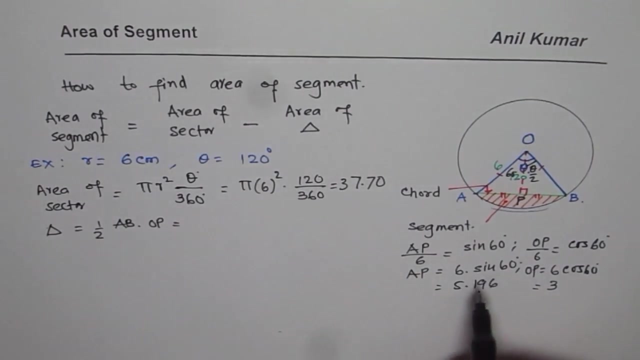 It is 5.196, let me write 196.. As far as OP is concerned, it is 6 times cos of 60 degrees, which is going to be half of this. so that is 3, right? So we have that. 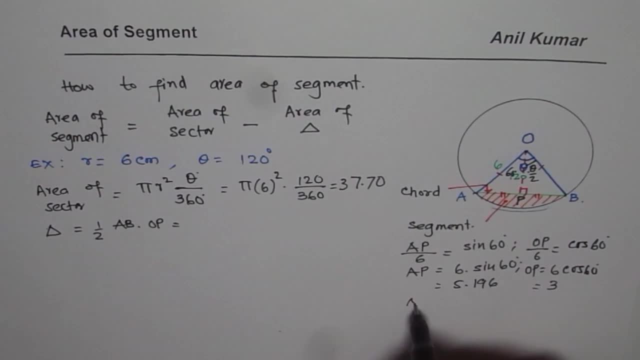 And we also know that AB is equals to 2 times AP, since P is the midpoint, 2 times AP, right? So it is, that is what we can use- 2 times 5.195.. So now we can write this formula here: 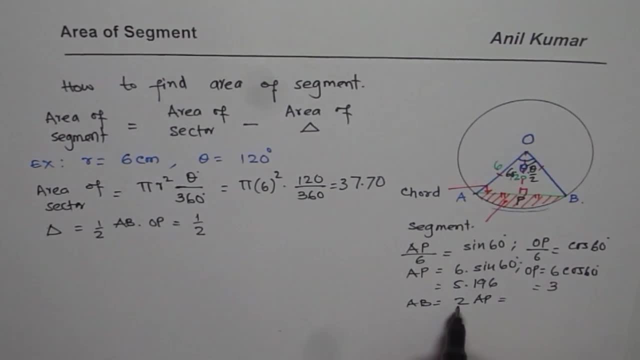 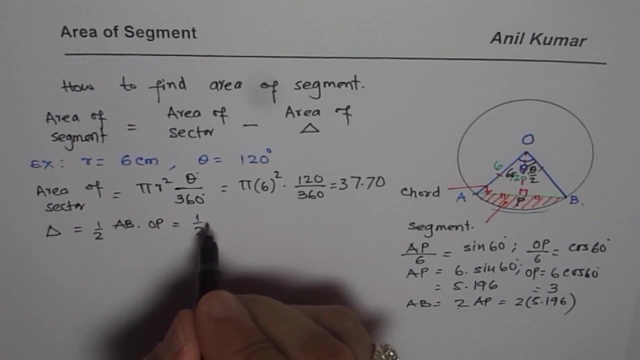 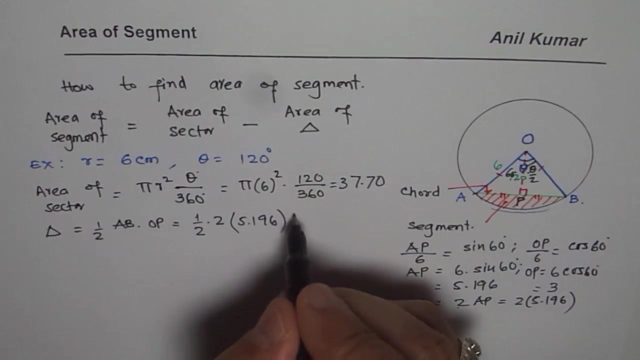 as area of the triangle is half AB. I am writing 2 times AP, which is 2 times 5.196,, is that okay? So times 2, times 5.196, and OP is 3 for us, is that okay? 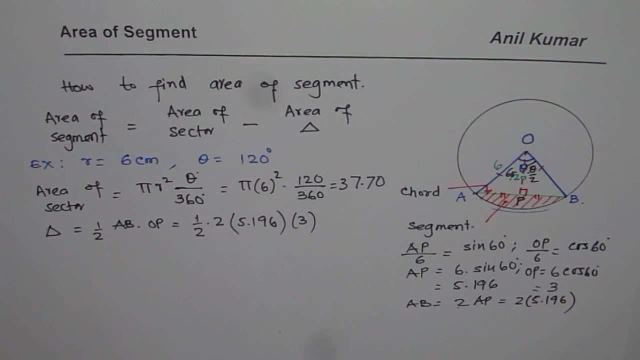 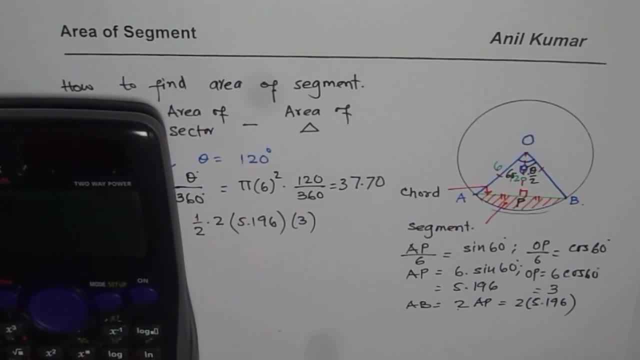 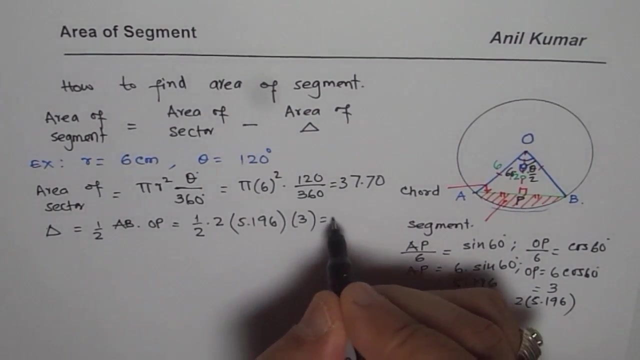 So we substitute all these values here, So 2 and 2 cancel, so we get 3 times 5.196, which is in decimals 15.58.. 15.588,, so let's say 5.9.. 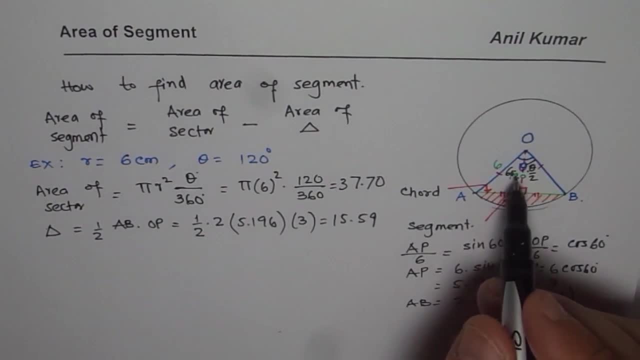 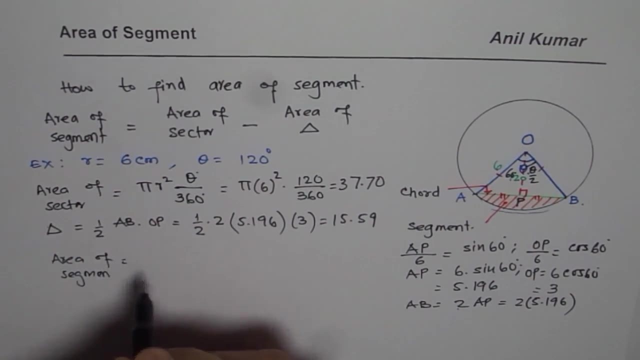 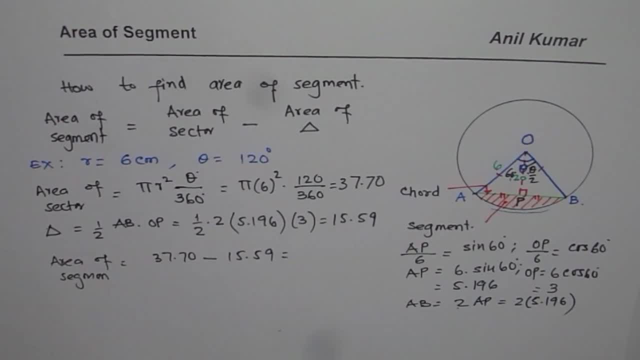 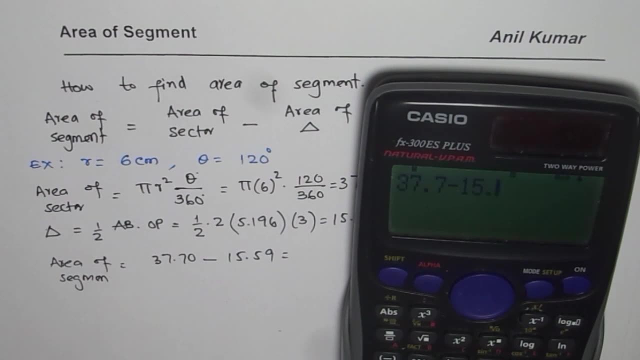